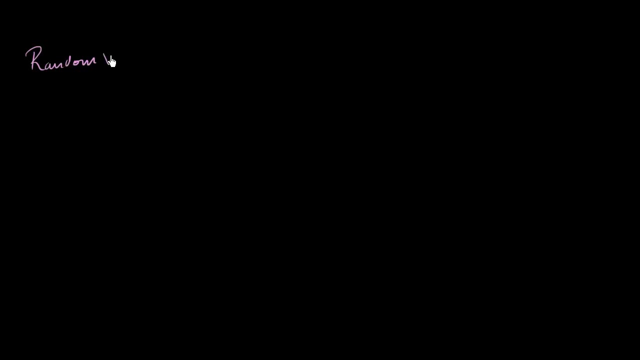 We already know a little bit about random variables. What we're going to see in this video is that random variables come in two varieties. You have discrete random variables and you have continuous random variables And discrete random variables. these are essentially random variables that can take on distinct or separate values. 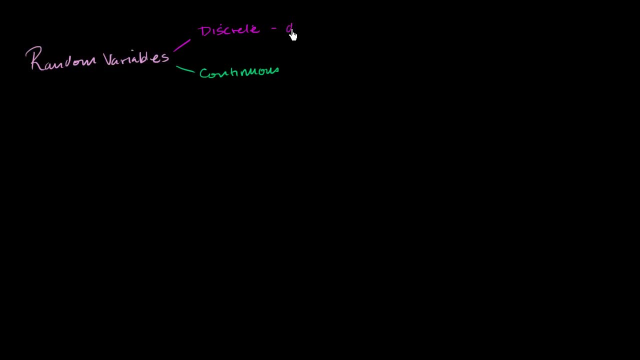 And we'll give examples of that in a second. So that comes straight from the meaning of the word discrete in the English language: Distinct or separate values While continuous, and I guess there's just another definition for the word discrete in the English language. 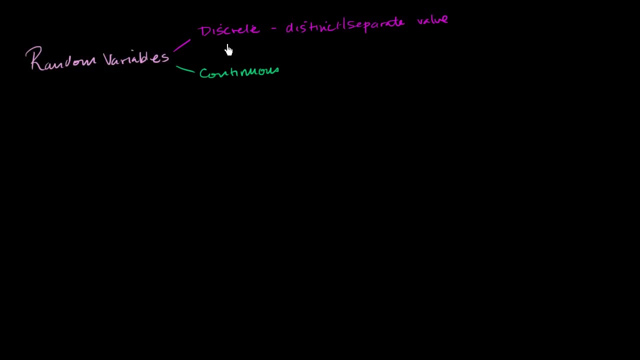 would be polite or not obnoxious or kind of subtle. That is not what we're talking about. We are not talking about random variables that are polite. We're talking about ones that can take on distinct values, And continuous random variables. they can take on any value in a range. 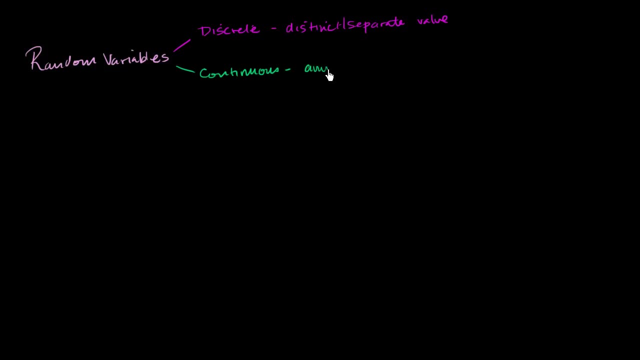 And that range could even be infinite. So any value in an interval. So with those two definitions out of the way, let's look at some actual random variable definitions, And I want to think together about whether you would classify them as discrete or continuous random variables. 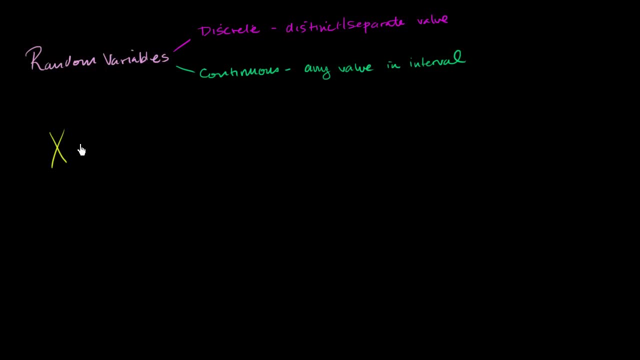 So let's say that I have a random variable capital X And it is equal to well. this is one that we covered in the last video. It's 1 if my fair coin is heads. It's a 0 if my fair coin is tails. 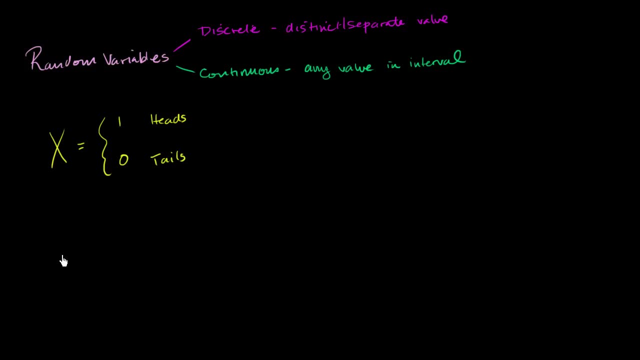 So is this a discrete or a continuous random variable? Well, this random variable right over here can take on distinct values. It can take on either one or it could take on a 0.. Another way to think about it is you can count the number of different values. 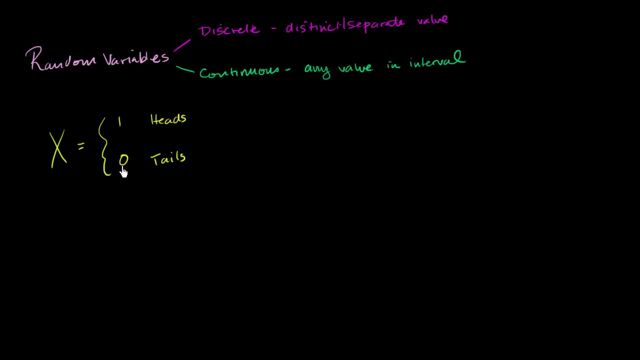 It can take on. This is the first value it can take on. This is the second value that it can take on. So this is clearly a discrete random variable. Let's think about another one. Let's define random variable Y as equal to the mass. 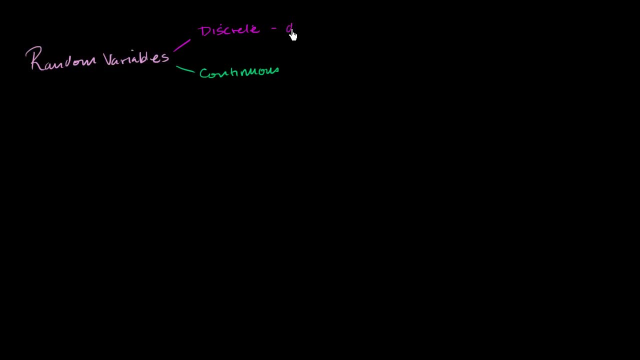 And we'll give examples of that in a second. So that comes straight from the meaning of the word discrete in the English language: Distinct or separate values While continuous, and I guess there's just another definition for the word discrete in the English language. 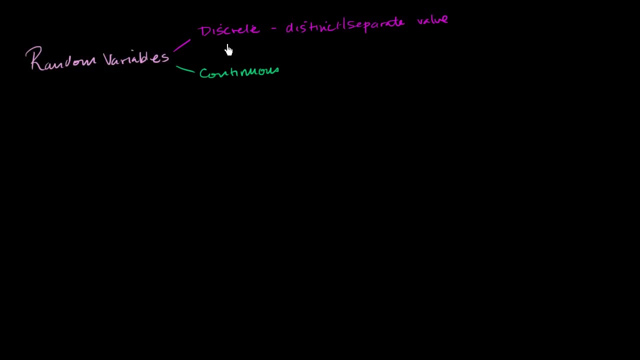 would be polite or not obnoxious or kind of subtle. That is not what we're talking about. We are not talking about random variables that are polite. We're talking about ones that can take on distinct values, And continuous random variables. they can take on any value in a range. 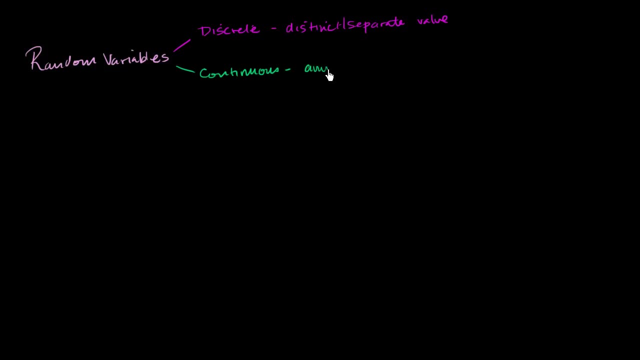 And that range could even be infinite. So any value in an interval. So with those two definitions out of the way, let's look at some actual random variable definitions, And I want to think together about whether you would classify them as discrete or continuous random variables. 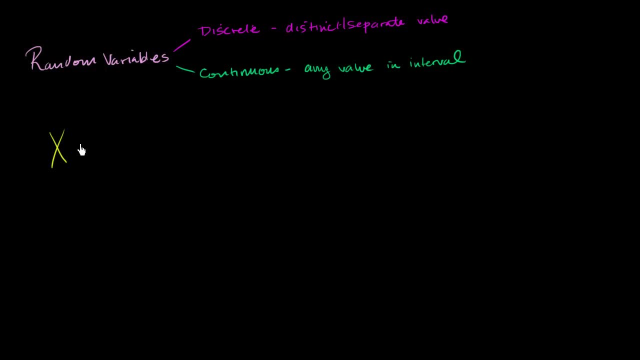 So let's say that I have a random variable capital X And it is equal to well. this is one that we covered in the last video. It's 1 if my fair coin is heads. It's a 0 if my fair coin is tails. 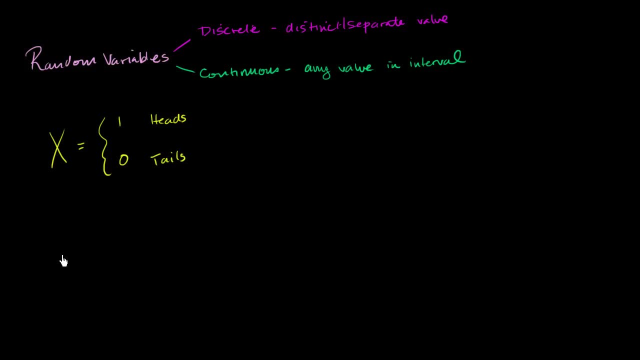 So is this a discrete or a continuous random variable? Well, this random variable right over here can take on distinct values. It can take on either one or it could take on a 0.. Another way to think about it is: you can count the number. 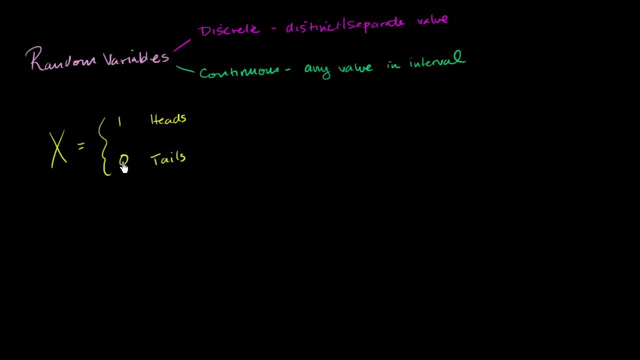 of different values it can take on. This is the first value it can take on. This is the second value that it can take on. So this is clearly a discrete random variable. Let's think about another one. Let's define random variable Y as equal to the mass. 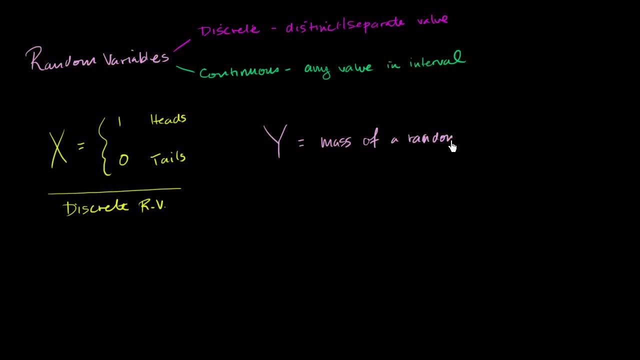 of a random animal. Animal selected at the New Orleans Zoo where I grew up: The Audubon Zoo At the New Orleans Zoo. The Audubon Zoo Y is the mass of a random animal selected at the New Orleans Zoo. 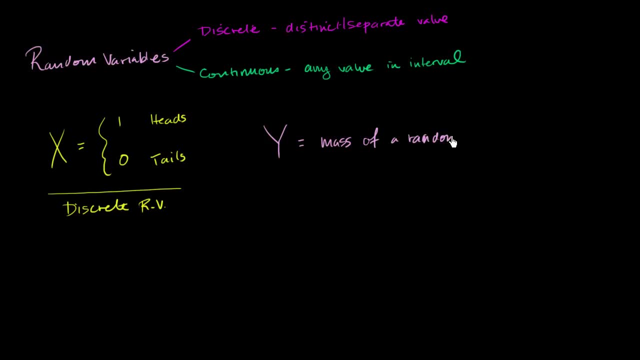 of a random animal Selected at the New Orleans Zoo where I grew up: The Audubon Zoo. At the New Orleans Zoo. The Audubon Zoo: Y is the mass of a random animal selected at the New Orleans Zoo. Is this a discrete random variable? 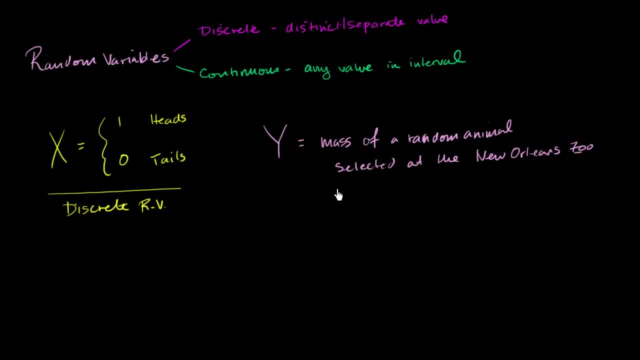 or a continuous random variable. Well, the exact mass- and I should probably put that qualifier here. I'll leave it at that. It's been added here just to make it really, really clear- The exact mass of a random animal or a random object. 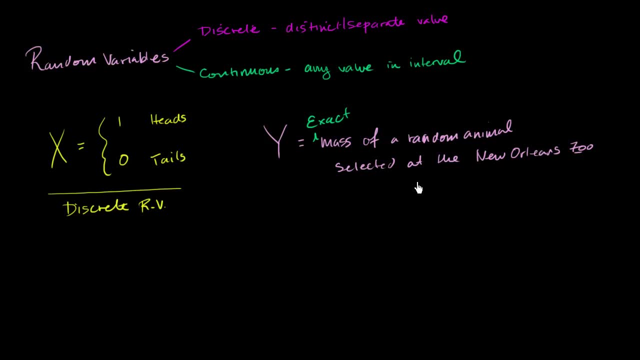 in our universe. it can take on any of a whole set of values. I mean, who knows exactly the exact number of electrons that are a part of that object right at that moment? Who knows the neutrons, the protons, the exact number? 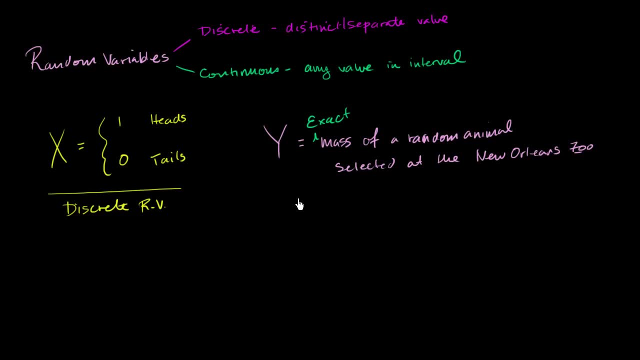 of molecules in that object or part of that animal exactly that moment. So that mass, for example, at the zoo, it might take on a value anywhere between well, maybe close to zero- There's no animal that has zero mass- But it could be close to zero if we're thinking about an ant. 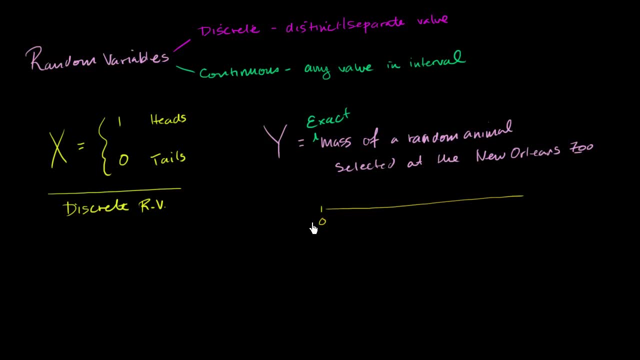 or we're thinking about a dust mite, or maybe, if you consider even a bacterium, an animal. I believe bacterium is the singular of bacteria, And it could go all the way. Maybe the most massive animal in the zoo is the elephant of some kind. 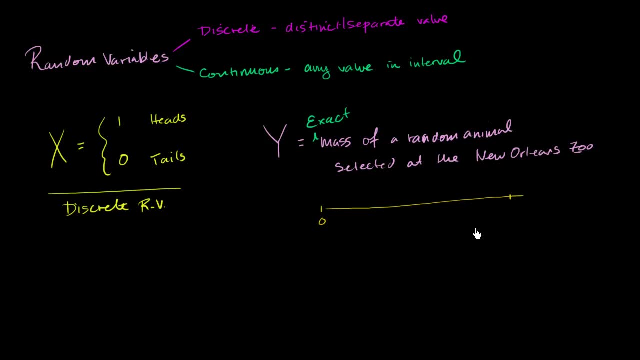 And I don't know what it would be in kilograms, but it would be fairly large. So maybe you can get up all the way to 3,000 kilograms, or probably larger, say 5,000 kilograms, I don't know what- the mass of a very heavy elephant. 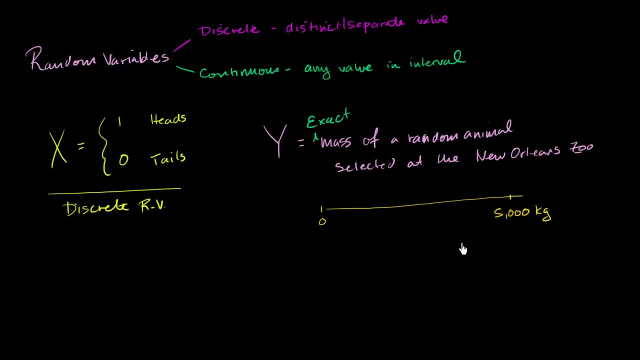 or a very massive elephant, I should say actually is. It may be something fun for you to look at, But any animal could have a mass anywhere in between. here It does not take on discrete values. You could have an animal that is exactly, maybe 120,000. 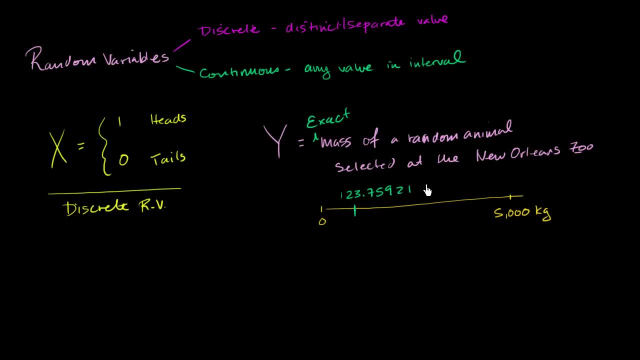 3.75921 kilograms, And even there that actually might not be the exact mass. You might have to get even more precise: 1, 0,, 7,, 3,, 2. And I think you get the picture. 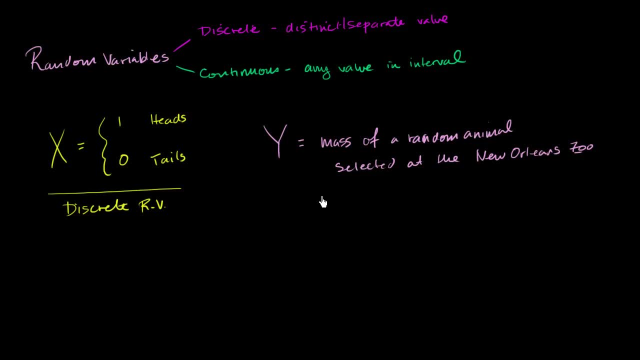 Is this a discrete random variable or a continuous random variable? Well, the exact mass- and I should probably put that qualifier here, I'll even add it here just to make it really clear- The exact mass of a random animal or a random object in our universe. 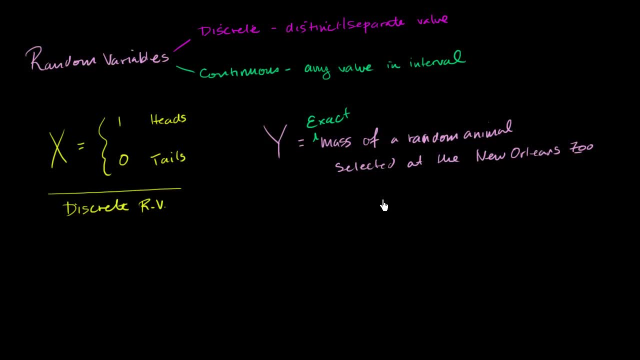 it can take on any of a whole set of values. I mean, who knows exactly the exact number of electrons that are a part of that object right at that moment? Who knows the neutrons, the protons, the exact number of molecules in that object or part of that animal? 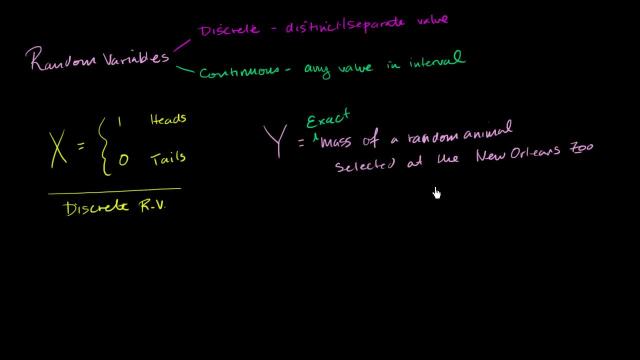 exactly at that moment, So that mass, for example at the zoo, it might take on. it might take on a value anywhere between well, maybe close to zero, close to zero. There's no animal that has zero mass, But it could be close to zero if we're thinking about an ant. 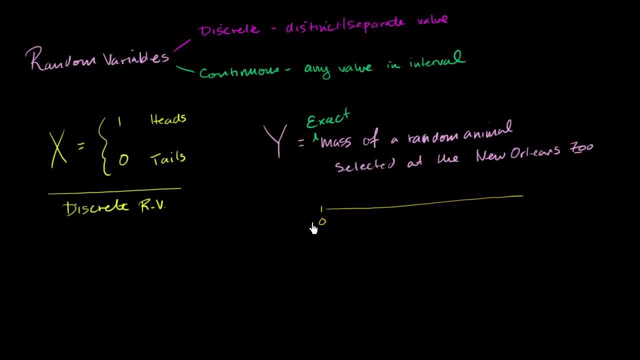 or we're thinking about a dust mite, or maybe, if you consider even a bacterium, an animal. I believe bacterium is the singular of bacteria, And it could go all the way. Maybe the most massive animal in the zoo is the elephant of some kind. And I don't know what it would be in kilograms, but it would be fairly large. So maybe you can get up all the way to 3,000 kilograms, or probably larger, say 5,000 kilograms, I don't know what- the mass of a very heavy elephant. 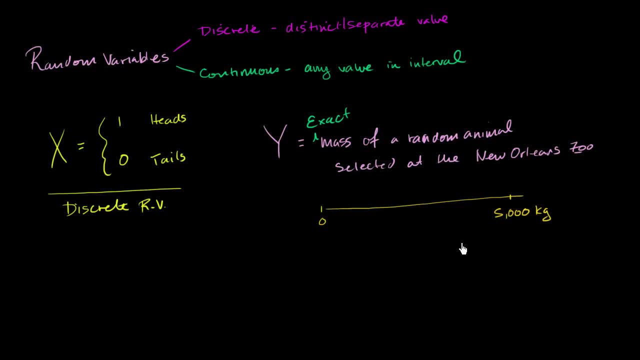 or a very massive elephant I should say actually is Maybe something fun for you to look at, But any animal could have a mass anywhere in between here It does not take on discrete values. You could have an animal that is exactly. 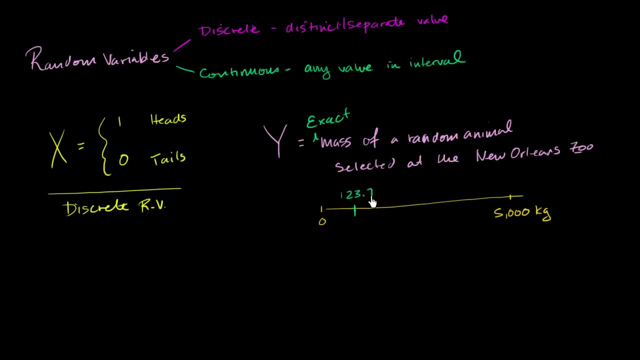 well, maybe It could be 123.75921 kilograms, And even there that actually might not be the exact mass. You might have to get even more precise: 1,, 0,, 7,, 3, 2.. 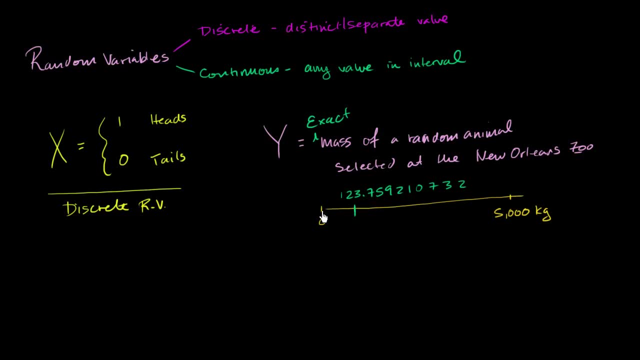 And I think you get the picture, Even though this is the way I've defined it now: a finite interval. you can take on any value in between. here There are not discrete values, So this one here is clearly a continuous random variable. 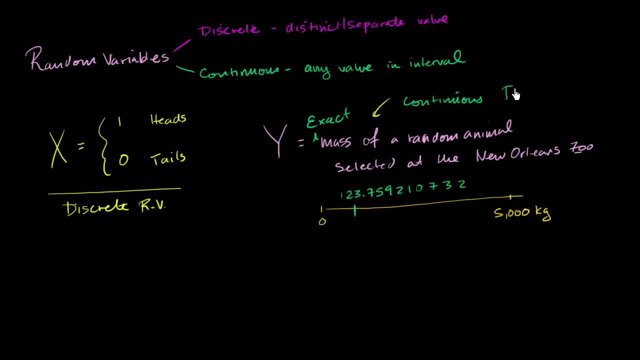 Continuous random variable. Let's think about another one. Let's think about, let's say, that random variable y, instead of it being this: let's say it's the year, the year that a random student in a class was born. Random student in a class was born. 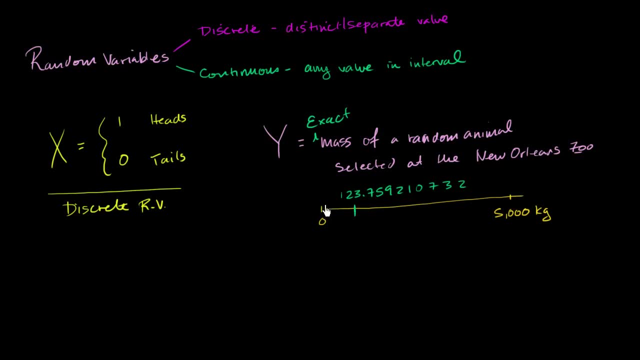 Even though this is the way I've defined it now- a finite interval. you can take on any value in between. here There are not discrete values. So this one here is clearly a continuous random variable. Continuous random variable. Let's think about another one. 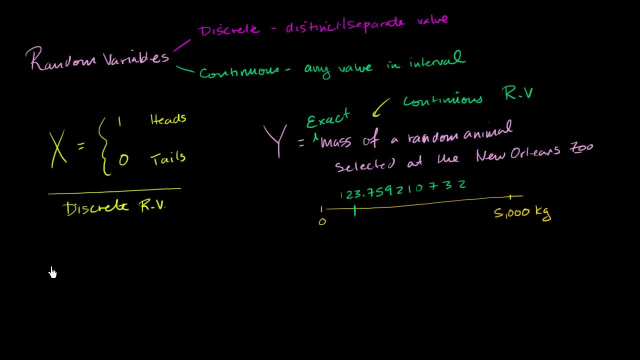 Let's think about, let's say, that random variable y instead of it being this. let's say, it's the year that a random student in a class was born. Random student in a class was born. Is this a discrete or a continuous random variable? 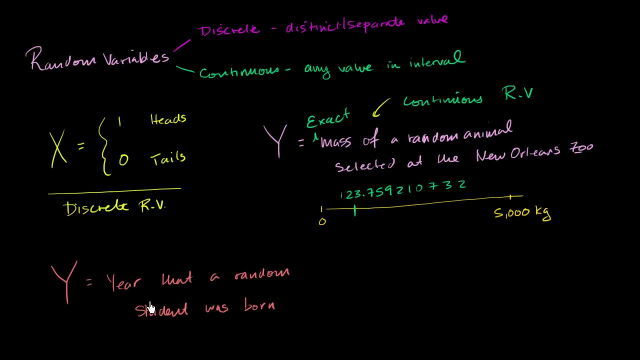 Well, that year, you literally can define it as a specific discrete year. It could be 1992, or it could be 1985, or it could be 2000 and 2001.. There are discrete values that this random variable. 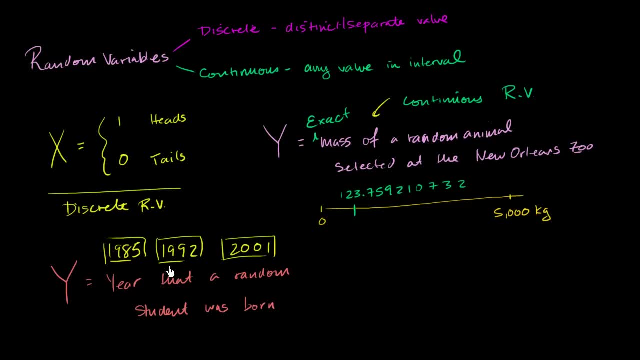 can actually take on. It won't be able to take on any value between, say, 2000 and 2001.. It'll either be 2000, or it'll be 2001, or 2002.. Once again, you can count the values it can take on. 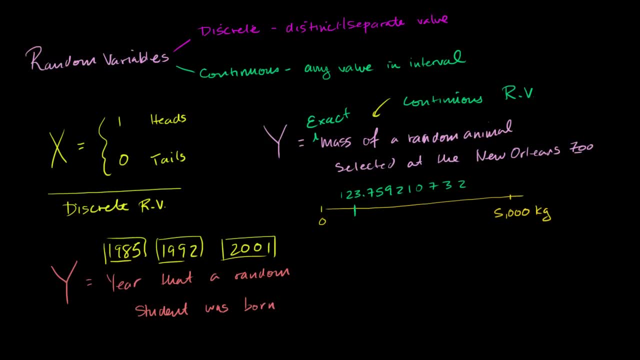 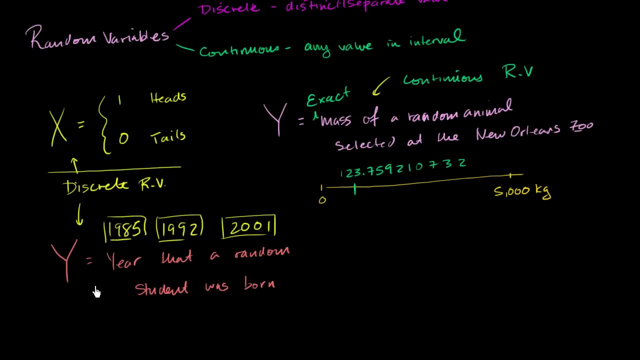 Most of the times that you're dealing with- as in the case right here- a discrete random variable- And let me make it clear: this one over here is also a discrete random variable. Most of the time that you're dealing with a discrete random variable, you're. 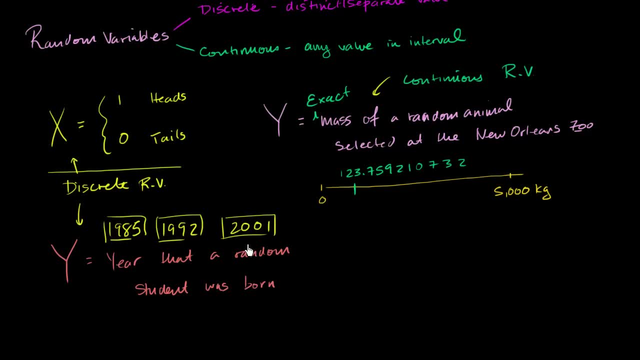 probably going to be dealing with a finite number of values, But it does not have to be a finite number of values. You can actually have an infinite potential number, a potential number of values It could take on as long as the values are countable. 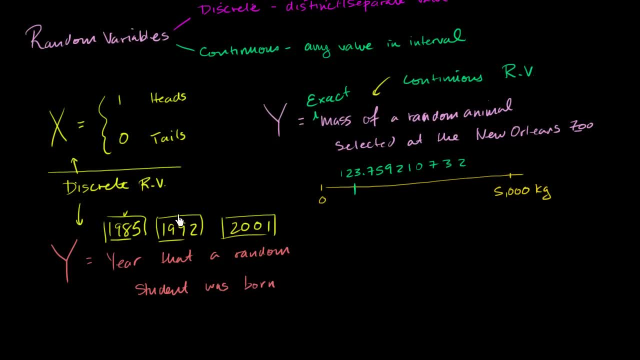 as long as you can literally say OK, this is the first value. it could take on the second, the third And you might be counting forever. But as long as you can literally list, and it could be even an infinite list. 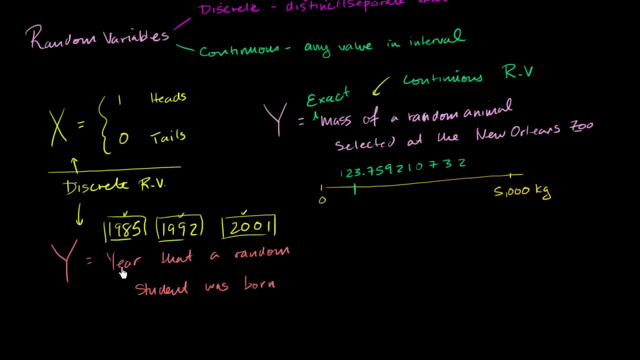 but if you could list the values that it could take on, then you're dealing with a discrete, random variable. Notice, in this scenario with the zoo, you could not list all of the possible masses, You could not even count them. You might attempt to, and it's a fun exercise. 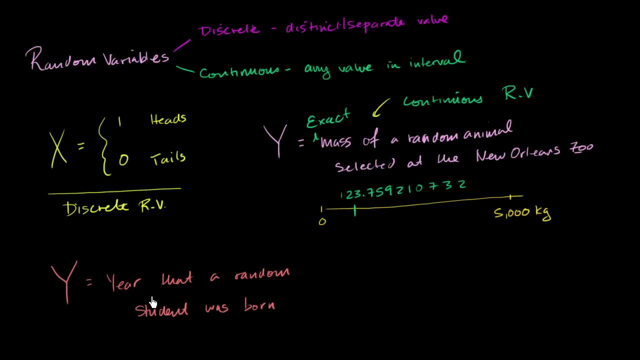 Is this a discrete Or a continuous random variable? Well, that year you literally can define it as a specific discrete year. It could be 1992.. Or it could be 1985. Or it could be 2000 and 2001.. 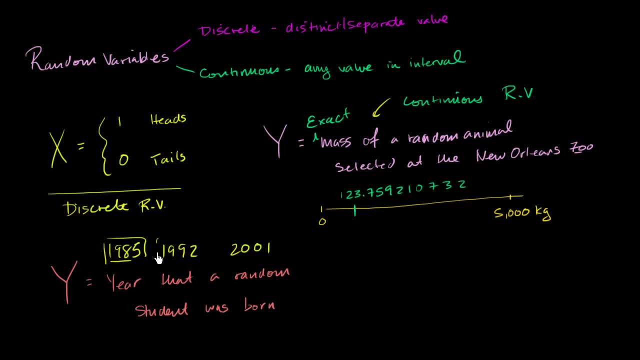 There are discrete values that this random variable can actually take on. It won't be able to take on any value between, say, 2000 and 2001.. It will either be 2000 or it will be 2001 or 2002.. 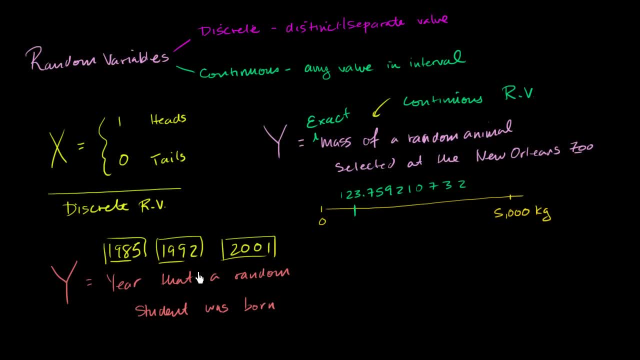 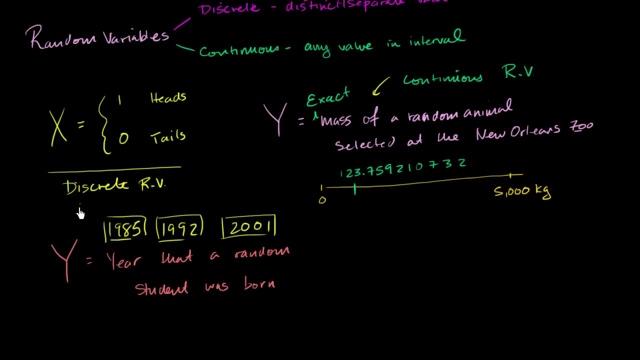 Once again, you can count the values. it can take on. Most of the times that you're dealing with, as in the case right here, a discrete random variable, And let me make it clear: this one over here is also a discrete random variable. 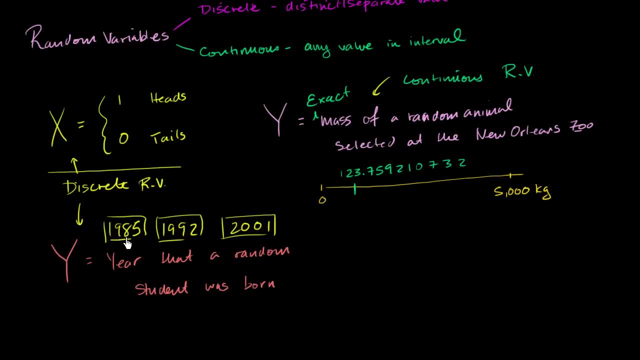 Most of the time that you're dealing with a discrete, random variable, you're probably going to be dealing with a finite number of values, But it does not have to be a finite number of values. You can actually have an infinite number of values. 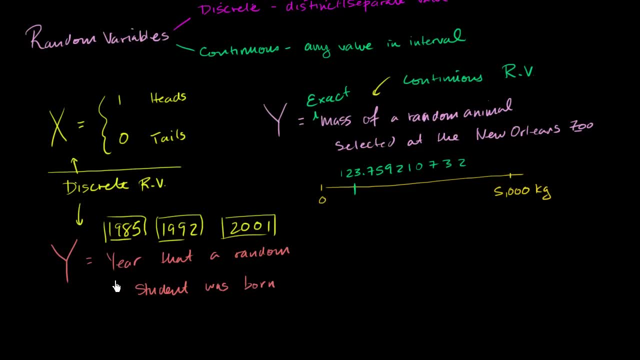 It may be infinite or finite, regardless a potential number of values that it could take on, as long as the values are countable, as long as you can literally say: okay, this is the first value it could take on, the second, the third, and you might be counting forever. 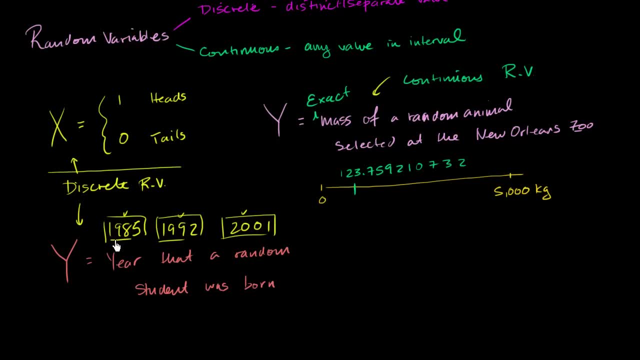 but as long as you can literally list- and it could be even an infinite list- but if you could list the values that it could take on, then you're dealing with a discrete, random variable. Notice, in this scenario with the zoo, you could not list all of the possible masses. 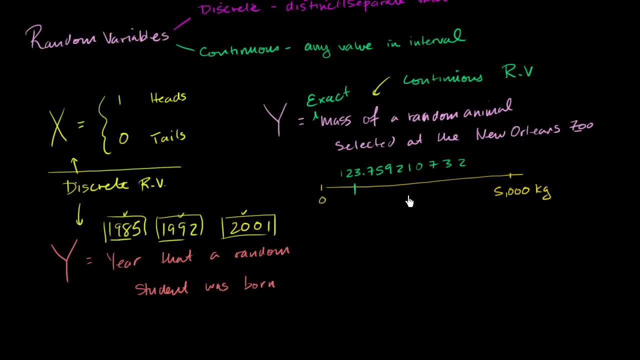 You could not even count them. You might attempt to- and it's a fun exercise to try at least once to try to list all of the values this might take on. You might say, okay, maybe you could take on 0.01,. 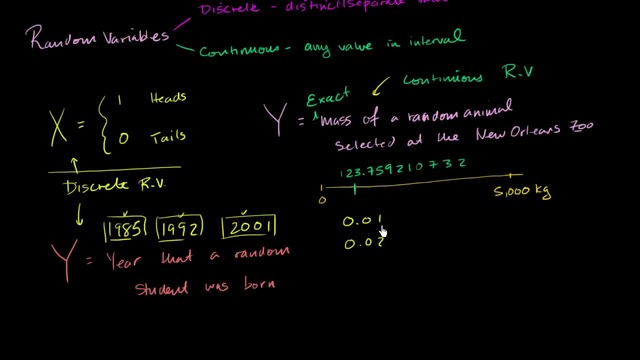 and maybe 0.02,. but wait, you just skipped an infinite number of values that it could take on, because it could have taken on 0.011,, 0.012, and even between those there's an infinite number of values it could take on. 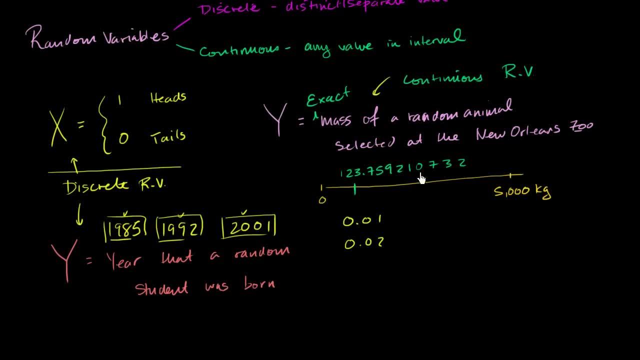 There's no way for you to count the number of values that a continuous random variable can take on. There's no way for you to list them. With a discrete random variable, you can count the values, You can list the values. Let's do another example. 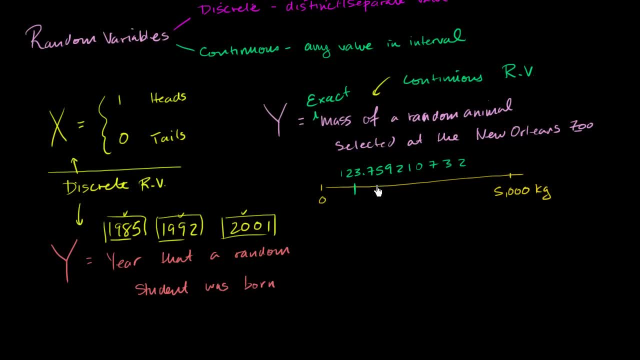 to try at least once to try to list all of the values this might take on. You might say, OK, maybe you could take on 0.01 and maybe 0.02.. But wait, you just skipped an infinite number of values. 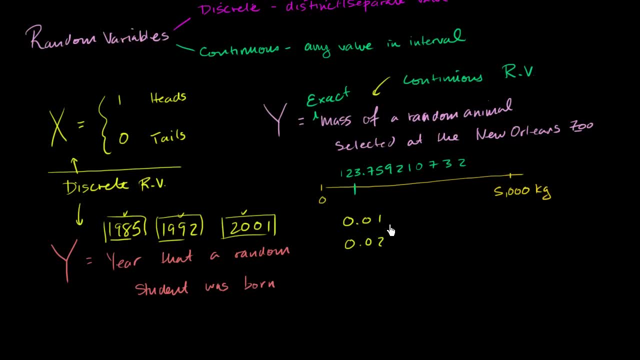 that it could take on, because it could have taken on 0.011,, 0.012. And even between those there's an infinite number of values it could take on. There's no way for you to count the number of values. 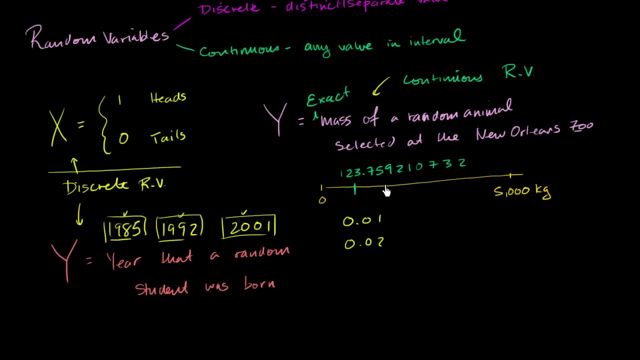 that a continuous random variable can take on. There's no way for you to list them With a discrete random variable. you can count the values, You can list the values. Let's do another example. Let's let random variable Z, capital Z. 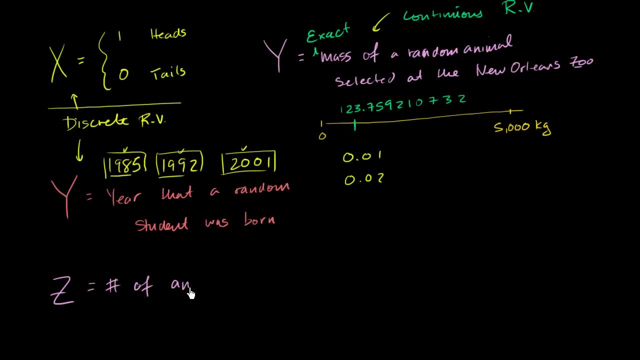 be the number of ants born tomorrow in the universe. Now you're probably arguing that there aren't ants on other planets, or maybe they're ant-like creatures, but they're not going to be ants as we define them. But how do we know? 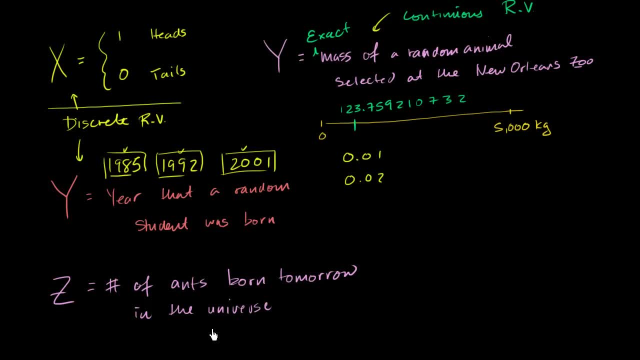 So number of ants born in the universe. Maybe some ants have figured out interstellar travel of some kind. So the number of ants born tomorrow in the universe, that's my random variable Z. Is this a discrete random variable or a continuous random variable? 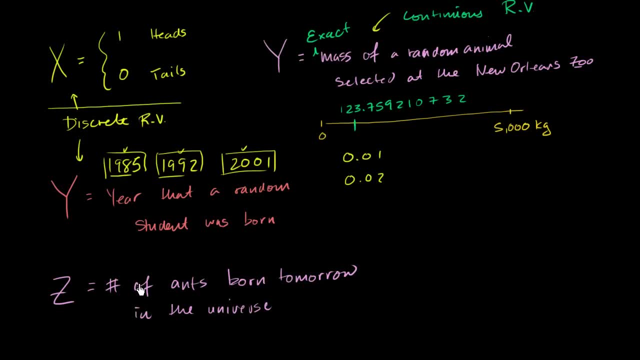 Well, once again we can count the number of values this could take on. This could be 1.. It could be 2.. It could be 3.. It could be 4.. It could be 5 quadrillion ants. It could be 5 quadrillion 1.. 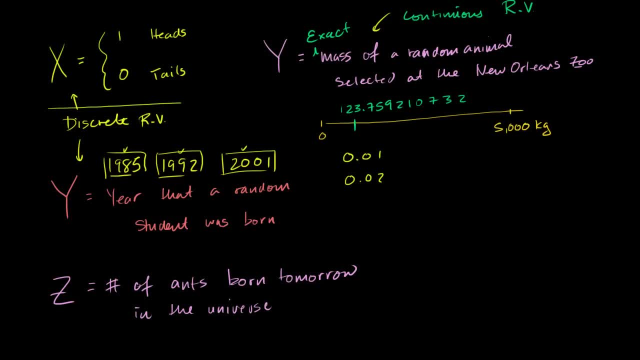 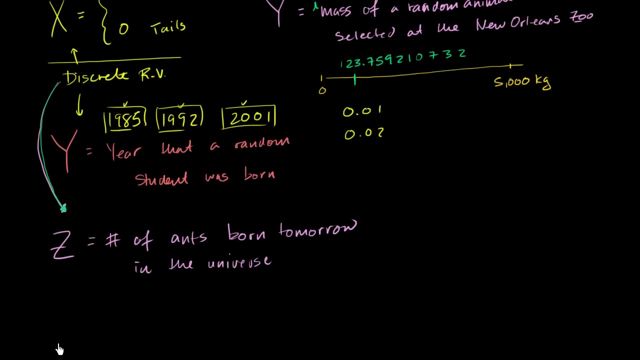 We can actually count the values. Those values are discrete. So once again, this right over here is a discrete random variable. This is fun, so let's keep doing more of these. Let's say that I have random variable x, So we're not using this definition anymore. 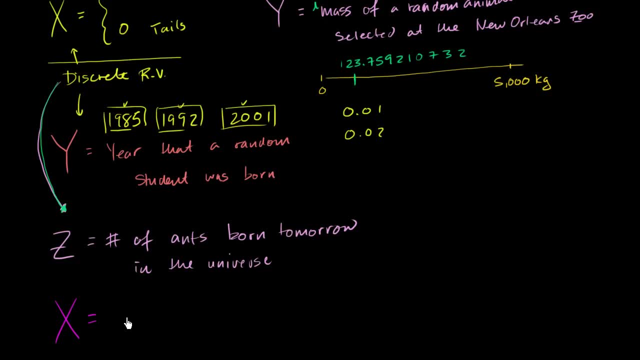 Now I'm going to define random variable x to be the winning time. Now, let me write it this way: The exact winning time for the men's men's 100 meter dash at the 2016 Olympics, 2016 Olympics. So the exact time that it took for the winner. who's? 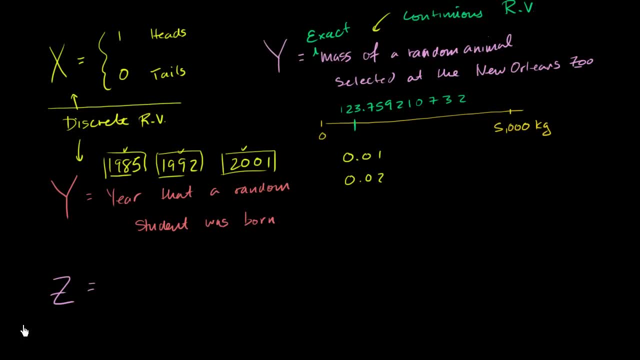 Let's let random variable Z, capital Z, be the number of ants born tomorrow in the universe. Now you're probably arguing that there aren't ants on other planets, or maybe they're ant-like creatures, but they're not going to be. 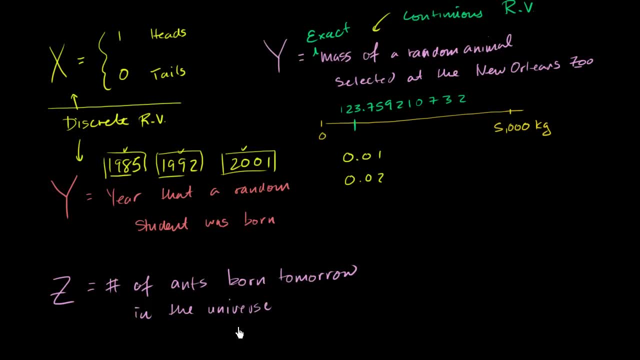 They're going to be ants as we define them. but how do we know So number of ants born in the universe? Maybe some ants have figured out interstellar travel of some kind. So the number of ants born tomorrow in the universe. 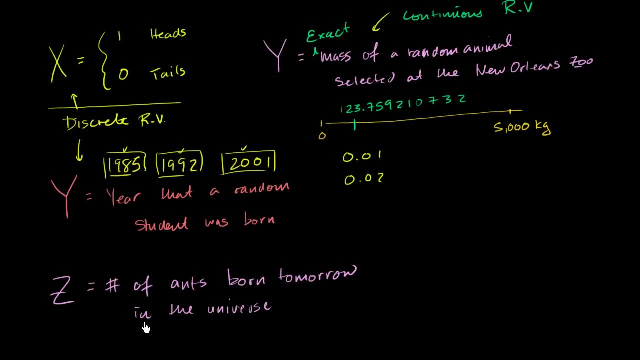 that's my random variable Z. Is this a discrete random variable or a continuous random variable? Well, once again we can count the number of values this could take on. This could be 1,, it could be 2,, it could be 3,, it could be 4,. 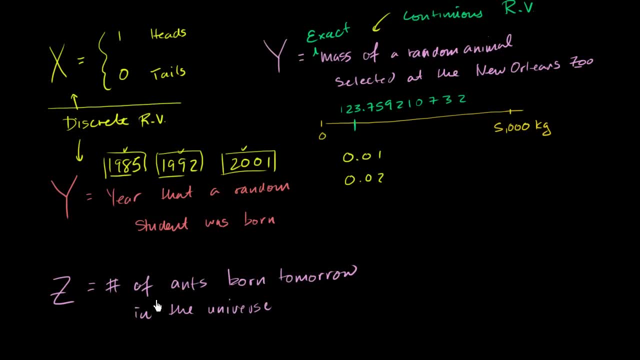 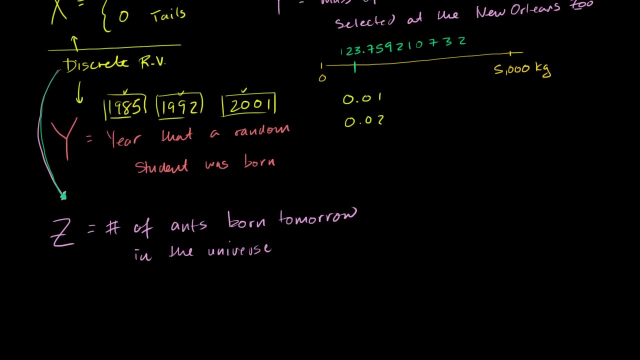 it could be 5 quadrillion ants. it could be 5 quadrillion 1.. We can actually count the values. Those values are discrete. So once again, this right over here is a discrete, random variable. This is fun, so let's keep doing more of these. 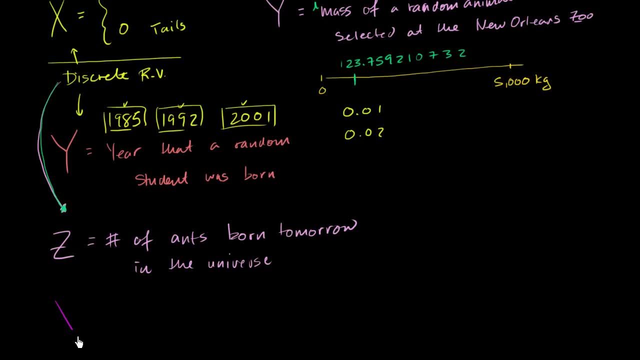 Let's say that I have random variable X, So we're not using this definition anymore. Now I'm going to define random variable X to be the winning time. Let me write it this way: the exact winning time. Winning time for the men's 100-meter dash. 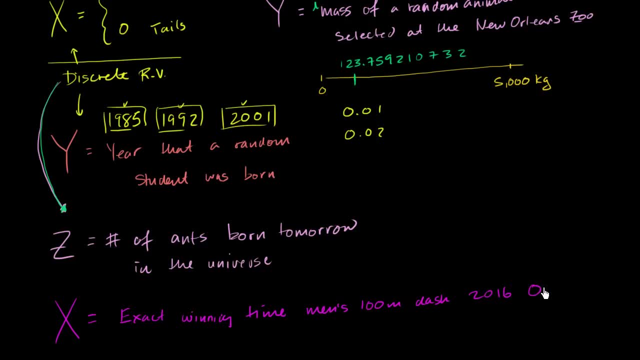 at the 2016 Olympics. So the exact time that it took for the winner, who's probably going to be Usain Bolt, but it might not be- Actually, he's aging a little bit- But whatever the exact winning time for the men's 100-meter. 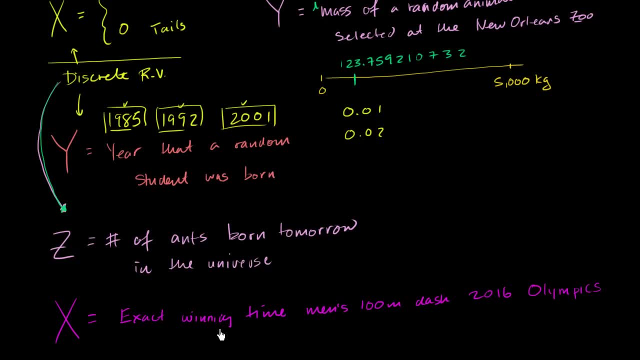 dash at the 2016 Olympics, And not the one that you necessarily see on the clock: The exact, The precise time that you would see at the men's 100-meter dash. Is this a discrete or continuous random variable? Well, the way I've defined it, and this one's. 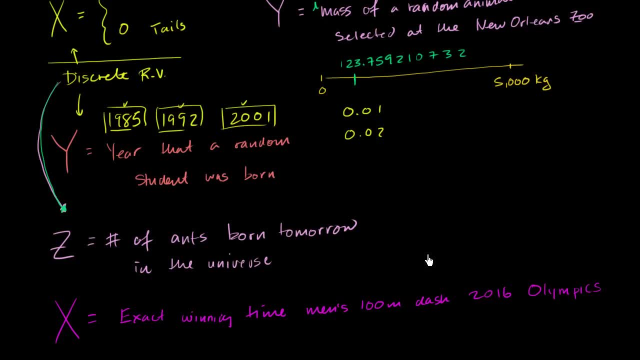 a little bit tricky Because you might say it's countable. You might say, well, it could be 9.56,, 9.56 seconds, or 9.57 seconds, or 9.58 seconds, And you might be tempted to believe that. 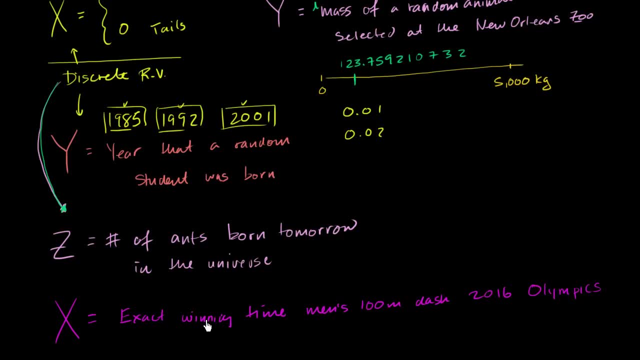 probably going to be Usain Bolt, but it might not be. Actually, he's aging a little bit, But whatever the exact winning time for the men's 100 meter dash at the 2016 Olympics- And not the one that you necessarily see on the clock- 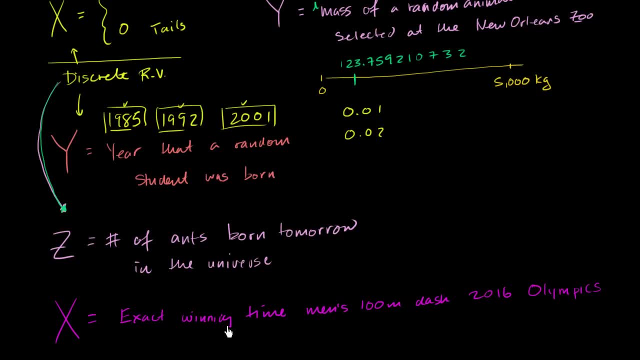 The exact, the precise time that you would see at the men's 100 meter dash. Is this a discrete or continuous random variable? Well, the way I've defined it- and this one's a little bit tricky Because you might say it's countable- 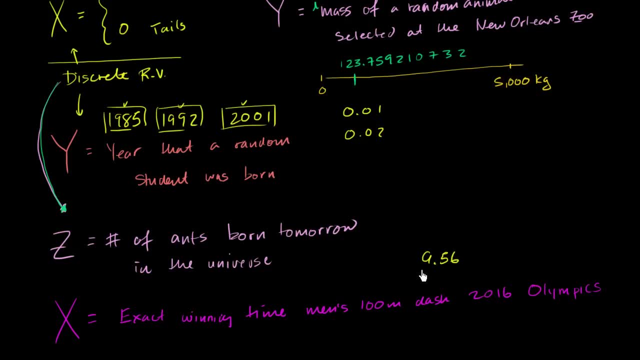 You might say: well, it could either be 9.56, 9.56 seconds or 9.57 seconds or 9.58 seconds. And you might be tempted to believe that Because when you watch the 100 meter dash at the Olympics, 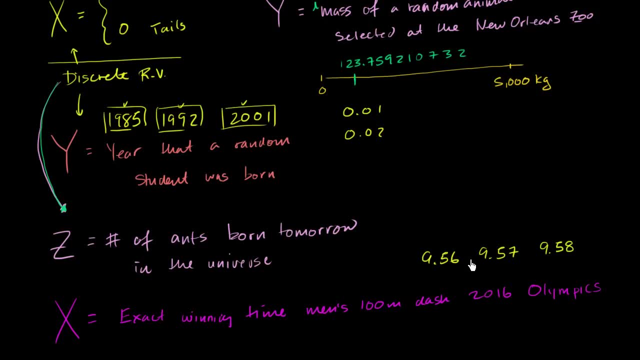 they measure it to the nearest hundreds, They round to the nearest hundreds. That's how precise their timing is. But I'm talking about the exact, The exact winning time, The exact number of seconds it takes for that person to from the starting gun to cross the finish line. 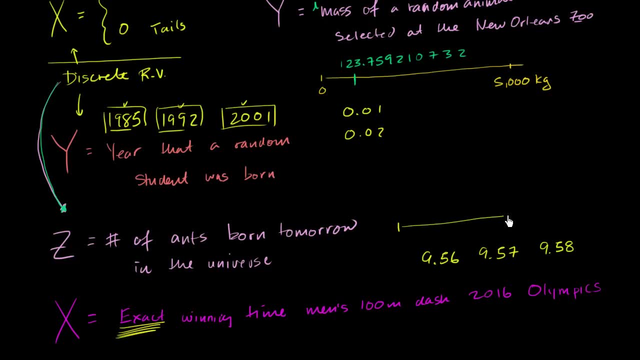 And there it can take on any value. It can take on any value between- well, I guess they're limited by the speed of light, But it could take on any value you could imagine, And it might be anywhere between 5 seconds, 5 seconds. 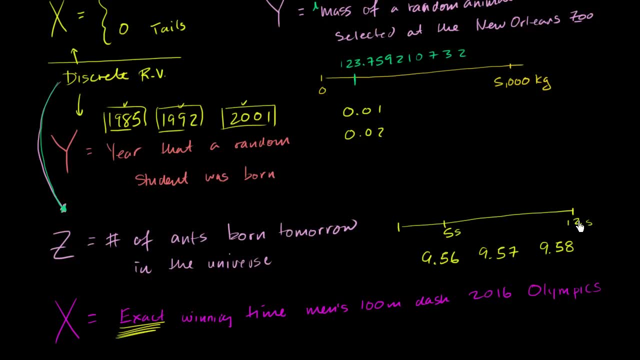 and maybe 12 seconds, And it could be anywhere in between. there It might not be 9.57.. That might be, That's what the clock says, But in reality the exact winning time could be 9.571.. Or it could be 9.572359.. 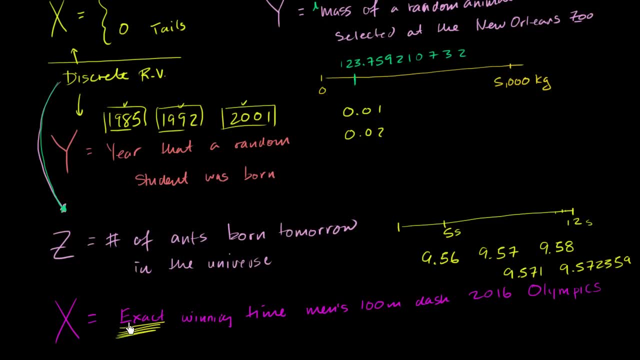 I think you see what I'm saying. The exact, precise time could be any value in an interval. So this right over here is a continuous random variable. Now, what would be the case, instead of saying the exact winning time, if instead I defined x? 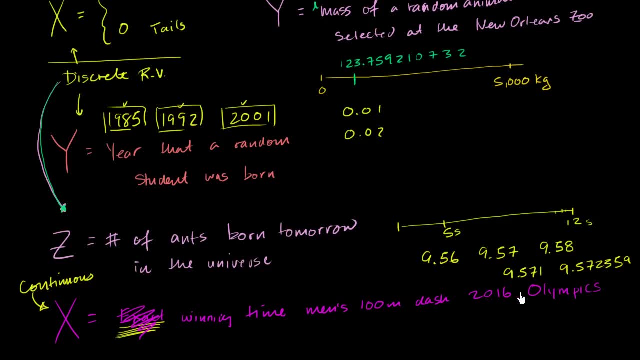 to be The winning time of the men's 100 meter dash at the 2016 Olympics, rounded to the nearest hundredth. Is this a discrete or a continuous random variable? So let me delete this. I've changed the random variable now. 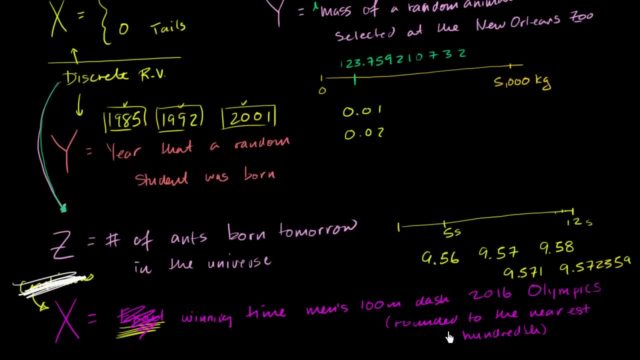 Is this going to be a discrete or continuous random variable? Well, now we can actually count the actual values that this random variable can take on. It might be 9.56.. It could be 9.57.. It could be 9.58.. 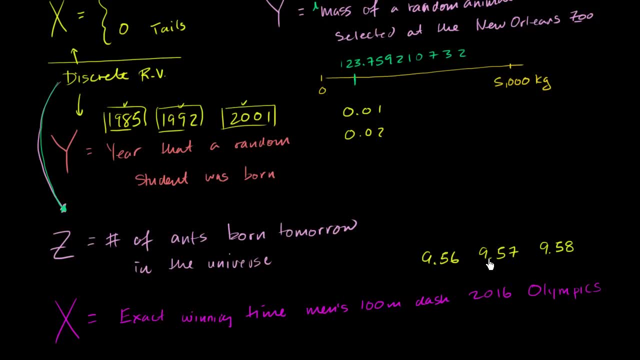 Because when you watch the 100-meter dash at the Olympics, they measure it to the nearest hundreds. They round, They measure the nearest hundreds. That's how precise their timing is. But I'm talking about the exact winning time, The exact number of seconds it takes for that person. 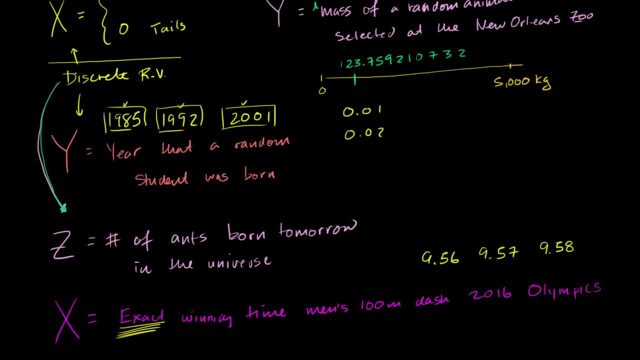 to from the starting gun to cross the finish line, And there it can take on any value. It can take on any value between- well, I guess they're limited by the speed of light, But it could take on any value you could imagine. 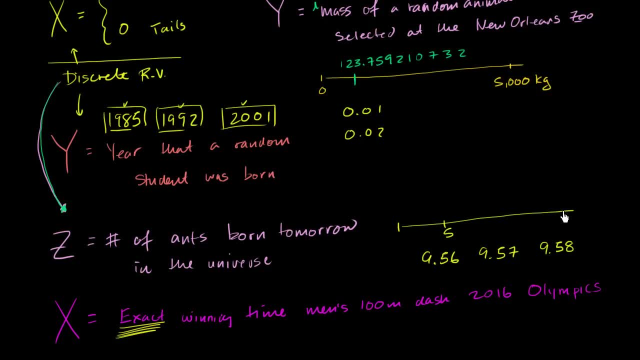 And it might be anywhere between 5 seconds and maybe 12 seconds And it could be anywhere in between. there It might not be 9.57.. That might be what the clock says, But in reality the exact winning time could be 9.571.. 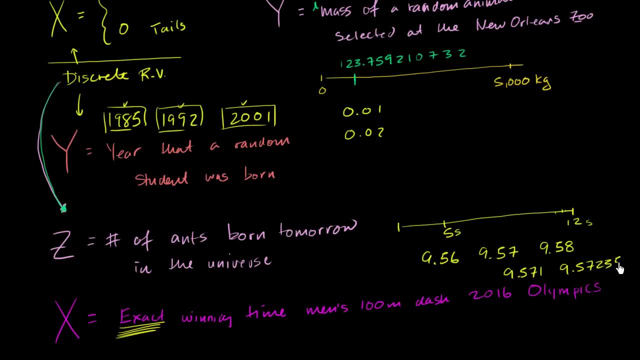 Or it could be 9.572359.. I think you see what I'm saying. The exact, precise time could be any value in an interval. So this right over here is a continuous random variable. Now what would be the case Instead of saying the exact winning time? 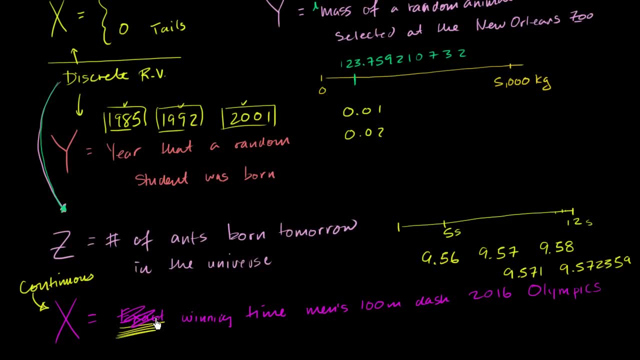 if instead, I defined x to be the winning time of the men's 100 meter dash at the 2016 Olympics, rounded to the nearest hundredth? Is this a discrete or a continuous random variable? So let me delete this. I've changed the random variable now. 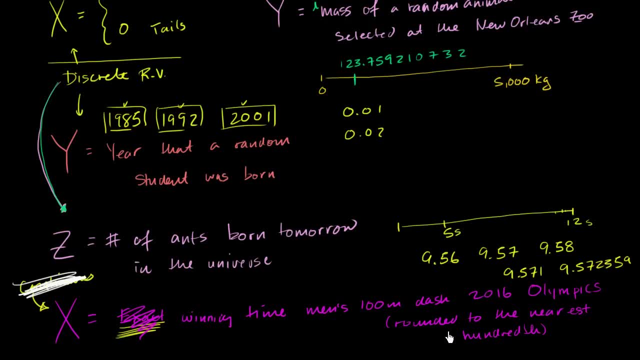 Is this going to be a discrete or continuous random variable? Well, now we can actually count the actual values that this random variable can take on. It might be 9.56.. It could be 9.57.. It could be 9.58.. 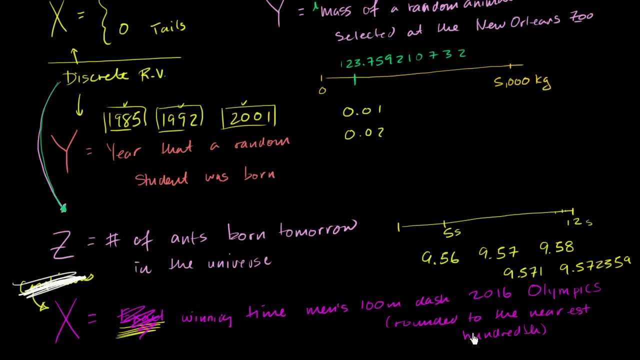 We can actually list them. So in this case, when we round it to the nearest hundredths, we can actually list the values. We are now just dealing with a discrete random variable. Anyway, I'll let you go there. Hopefully this gives you a sense of the distinction. 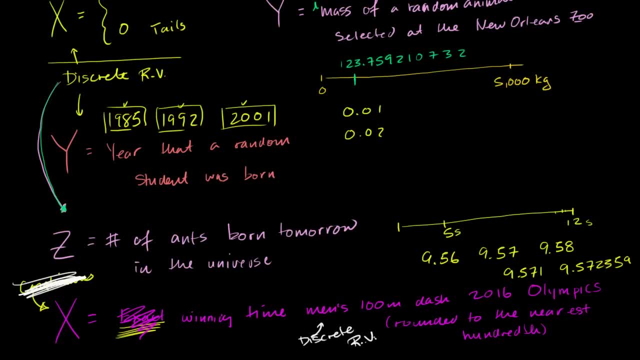 between discrete and continuous random variables.